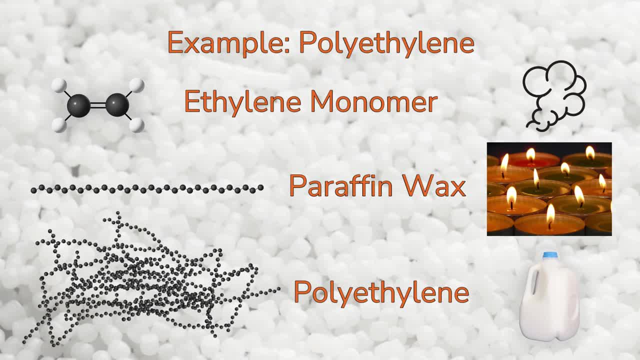 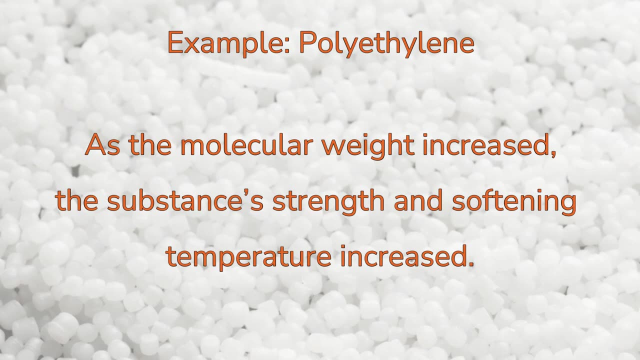 It is a ductile solid at room temperature and has a melting temperature of over 200 degrees Fahrenheit. While these three substances are made up of the same monomer, they behave very differently from each other. In this example, as the molecular weight increased, the substance's strength and softening temperature increased because of the stronger intermolecular bonds between the molecules. 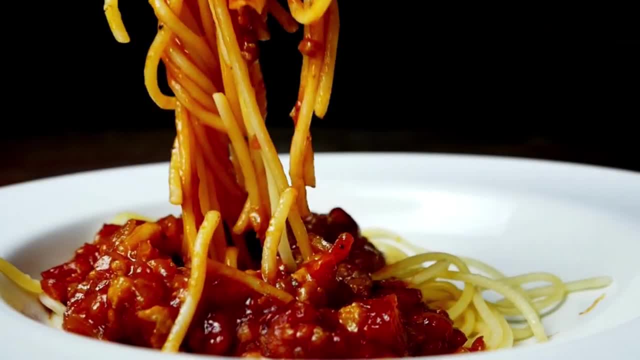 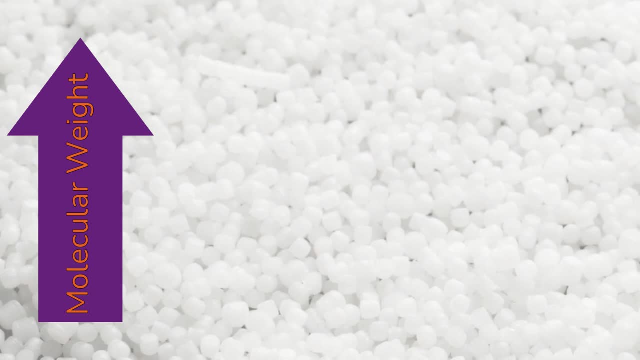 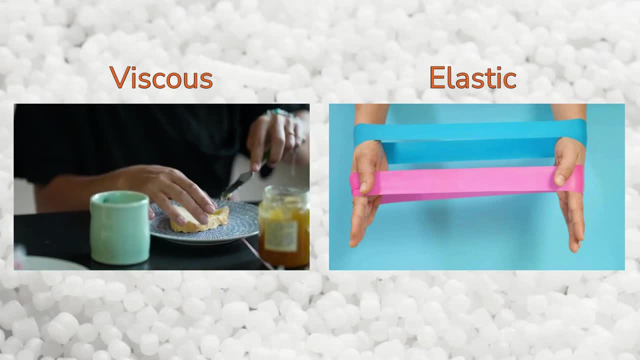 As the molecular weight of a polymer molecule increases, the material exhibits increased tensile strength, elongation and strength. As the molecular weight of a polymer molecule increases, the material exhibits increased tensile strength, elongation and strength. Biscus materials resist shear flow and strain linearly with time as stress is applied. 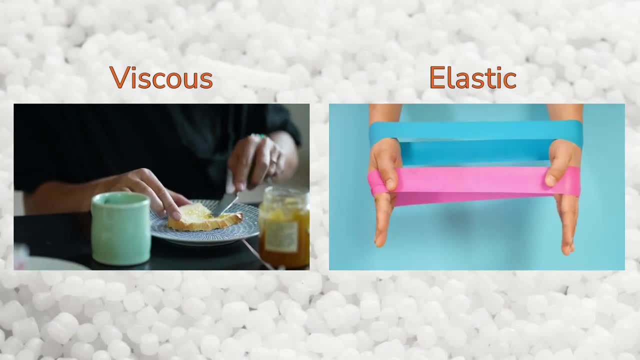 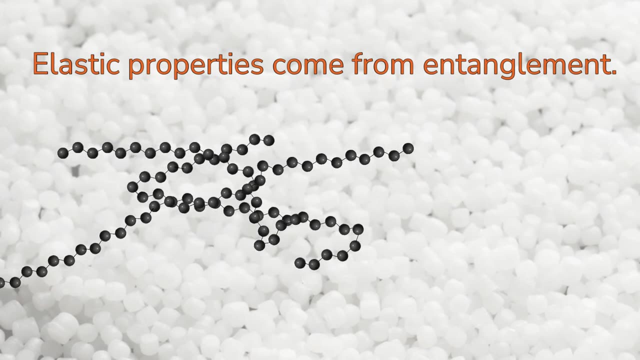 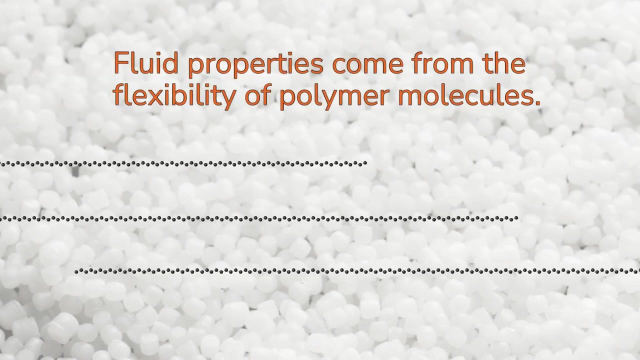 whereas elastic materials will strain when stressed quickly and return to their original state once the stress is removed, Polymer molecules, which are long chains, can temporarily connect or entangle with each other, which causes the elastic properties, and, on the other hand, due to their flexibility, they could easily slide past each other, which causes the fluid properties. 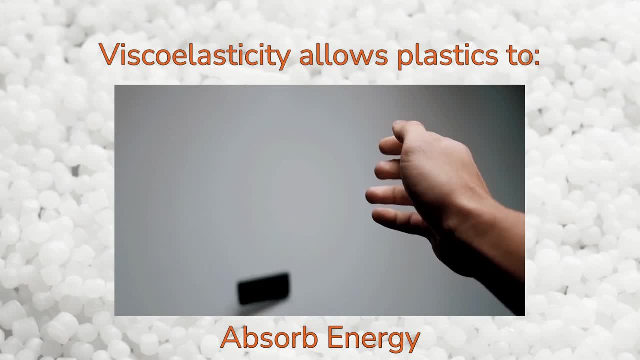 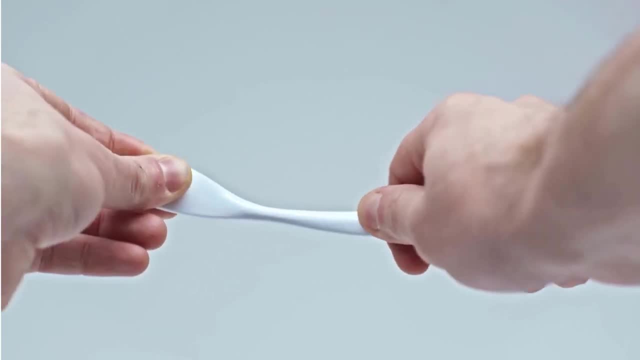 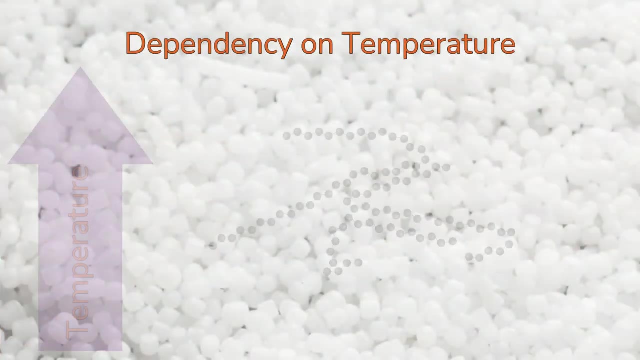 Viscoelasticity gives polymeric materials the ability to absorb energy, flex and spring back into shape without breaking. However, if the yield stress of a polymer is exceeded, the material will permanently deform. The behavior of viscoelastic materials is dependent on temperature. 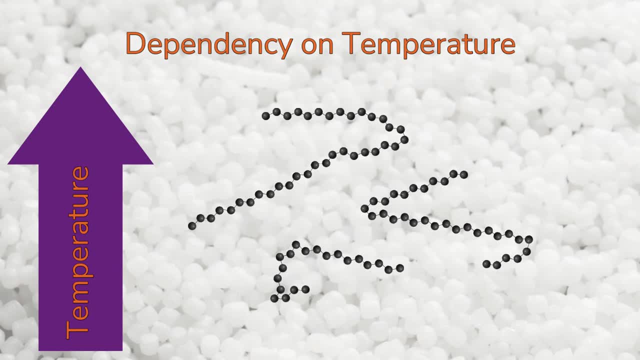 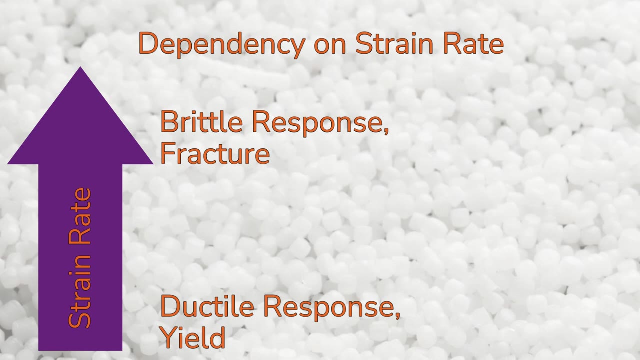 As the temperature increases, polymer chains move further apart, increasing the free volume between molecules and increasing the kinetic energy of the polymer chains. This allows them to slide past one another and disentangle more easily. Viscoelastic materials behavior is also dependent on strain rate. 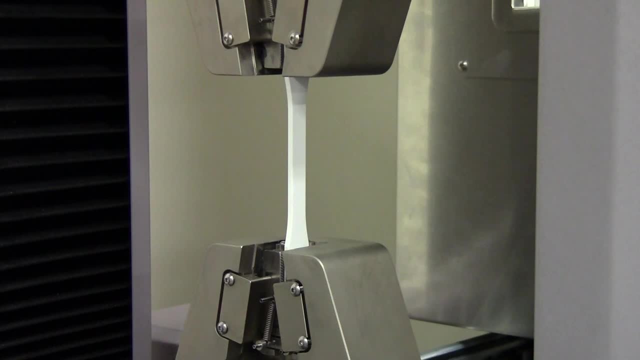 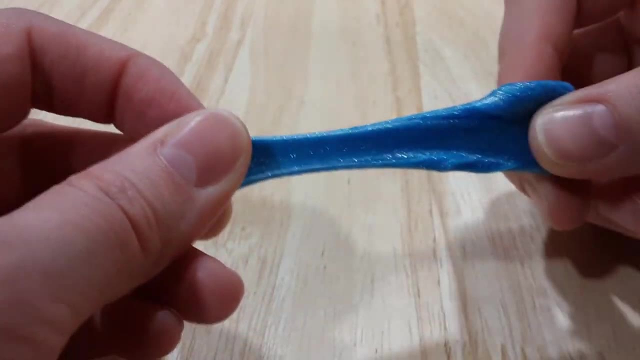 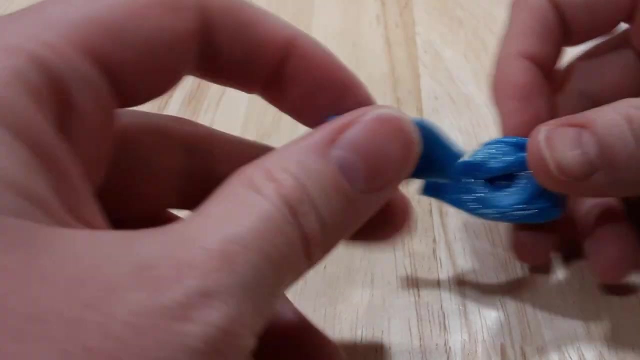 When the strain rate is fast, polymer chains do not have enough time to rearrange or undergo yielding, so instead they will disentangle. Elevated strain rates result in a ductile to brittle transition, and this is why pulling on Silly Putty slowly results in plastic deformation, while pulling on it quickly results in the. 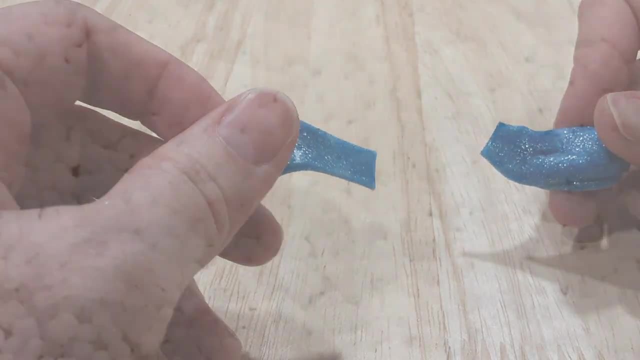 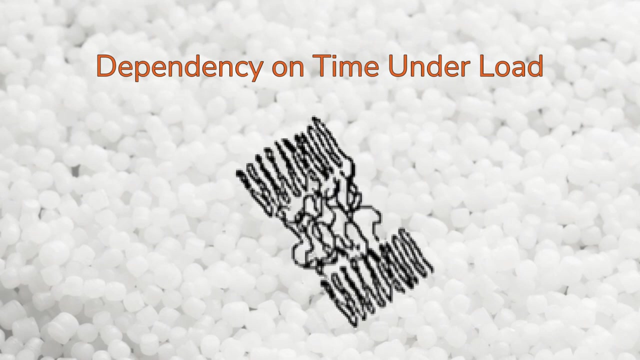 Silly Putty snapping in half, which is a brittle transition Material behavior. Time under load also determines how viscoelastic materials will behave Over time. when a force is applied to a part, polymer chains can rearrange and disentangle. 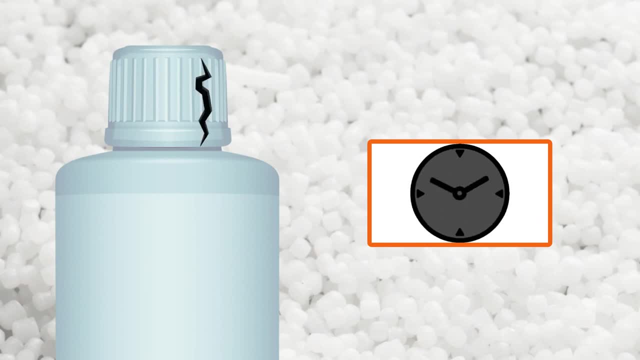 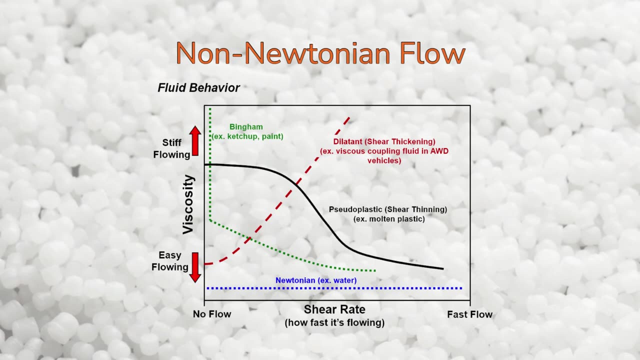 This is why plastic lids that are screwed tightly onto a bottle may crack if left untouched for a long time. In addition to having viscoelastic properties, polymers also exhibit non-Newtonian flow. This means that the viscosity of a molten polymer changes depending on the shear rate. 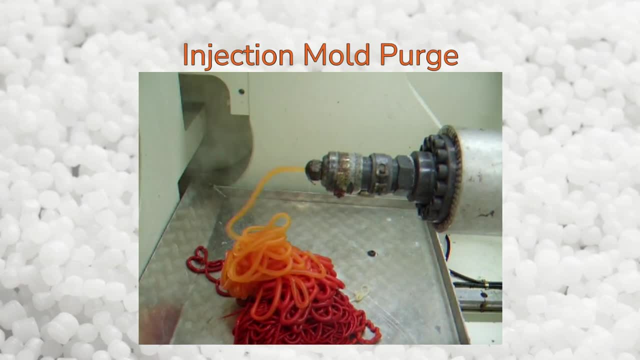 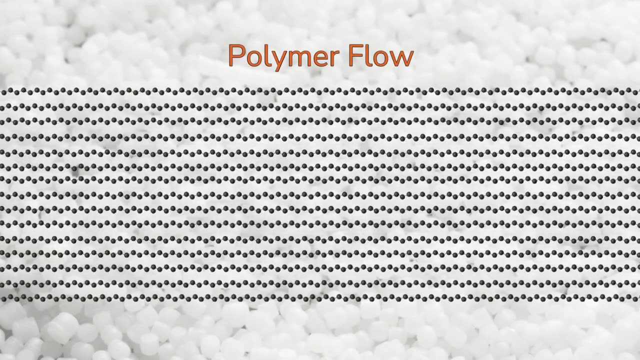 When a molten polymer changes, the viscosity of the molten polymer changes. When a molten polymer flows quickly, such as during the injection molding process, the polymer chains align like dry spaghetti noodles in a box. This allows them to slide past each other more easily. 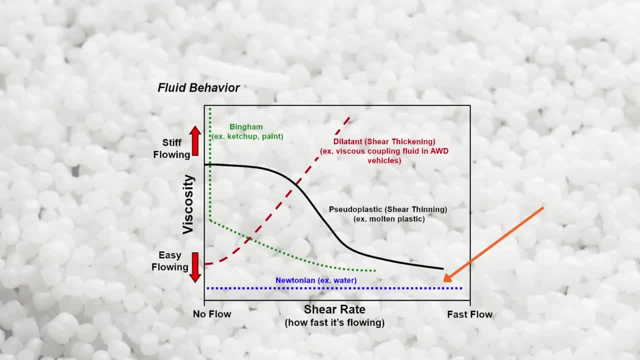 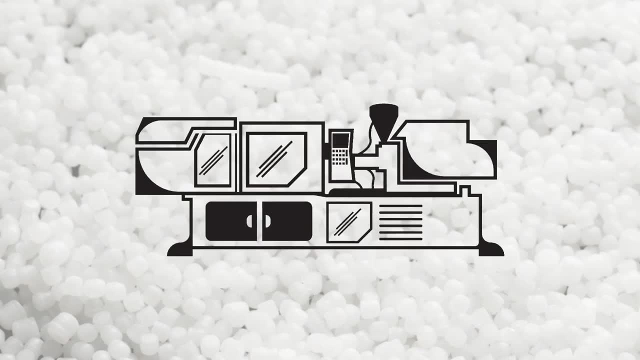 For a Newtonian fluid, like water, its viscosity is independent of shear rate. For a non-Newtonian fluid, its viscosity will change as the shear rate changes. This property makes thermoplastics injection moldable, so parts like Legos, car bumpers. 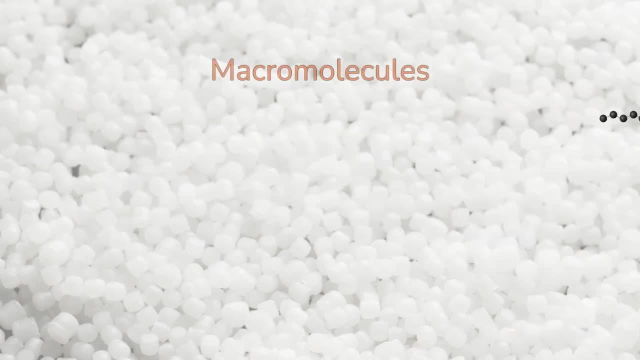 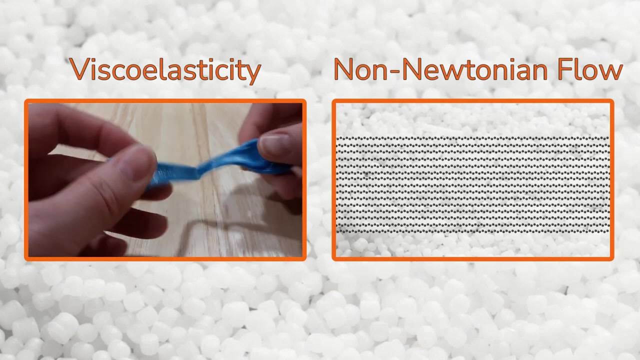 light switch, wall plates and many others can be mass produced. In this video, we learned that polymer chains are macromolecules that are made up of multiples of simpler chemical units called monomers. Their long fiber-like shape gives polymeric materials unique properties such as viscoelasticity. 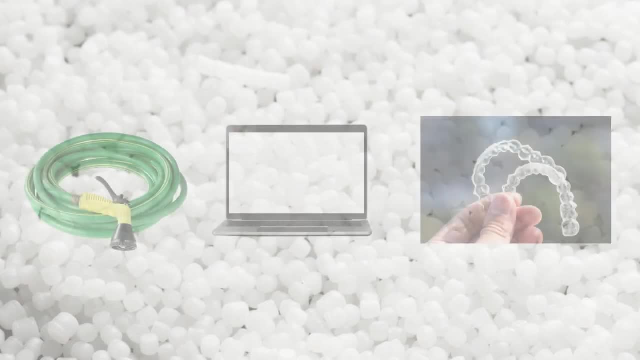 and non-Newtonian flow. These properties allow us to manufacture plastic parts that would not be possible to make out of metal, wood, glass or other readily available materials. In the next video, we'll discuss the differences between two categories of polymers. 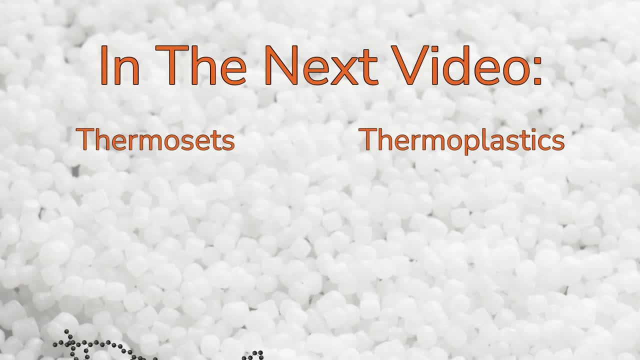 In this video, we learned that polymer chains are macromolecules that are made up of multiples of simpler chemical units called monomers. In this video, we learned that polymers are macromolecules that are made up of multiple categories of polymeric materials: thermosets and thermoplastics. 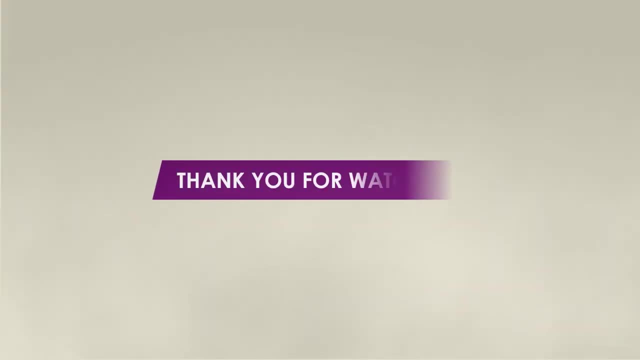 In this video, we learned that polymers are macromolecules that are made up of multiple categories of polymeric materials: thermosets and thermoplastics. Thank you for watching. If you enjoyed this video, please hit the like button to let us know and comment below.